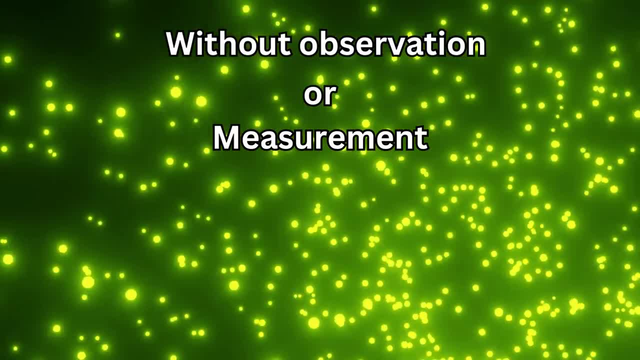 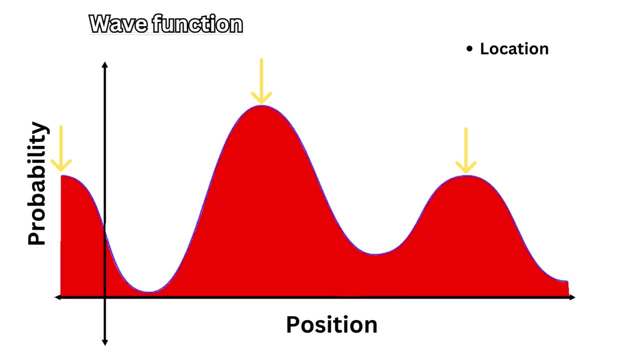 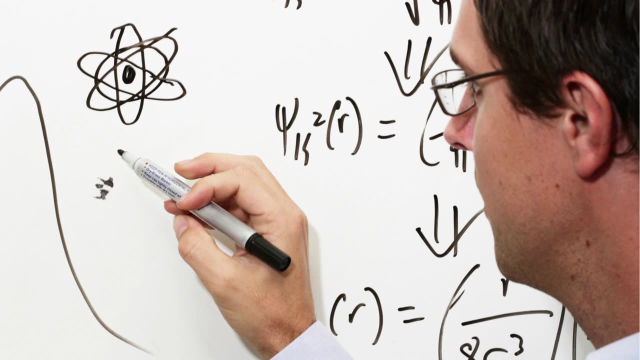 Think of the wave function as being similar to a probability wave or chance wave, Without observation or measurement. small particles like electrons lack a fixed position or state. A wave can be in sort of like a dispersed wave of potential. Although the wave function is only a mathematical probability, it demonstrates as a wave. 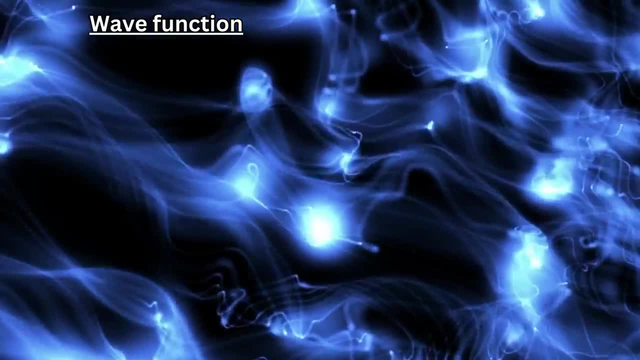 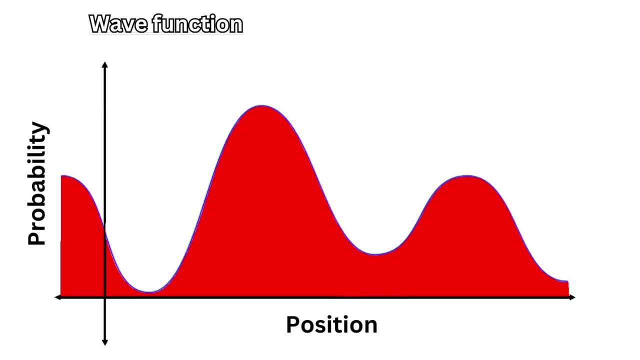 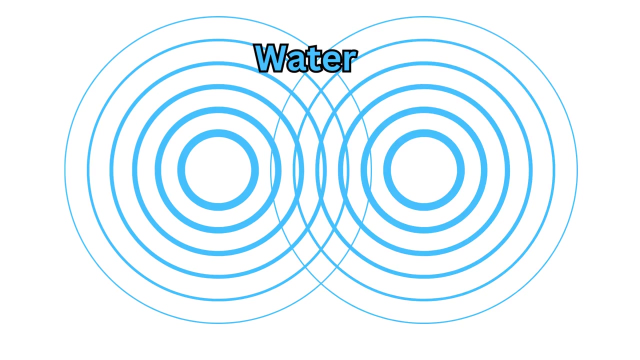 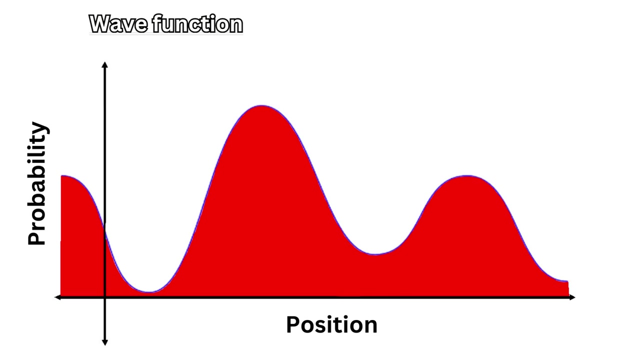 It may disperse round itself and even arrange itself in patterns of light and darkness. What's remarkable is that this probability wave can act in a manner reminiscent of how waves in water actually behave. In water, overlapping waves can produce patterns of high and low points. this is similar to how probability waves of particles can form patterns. 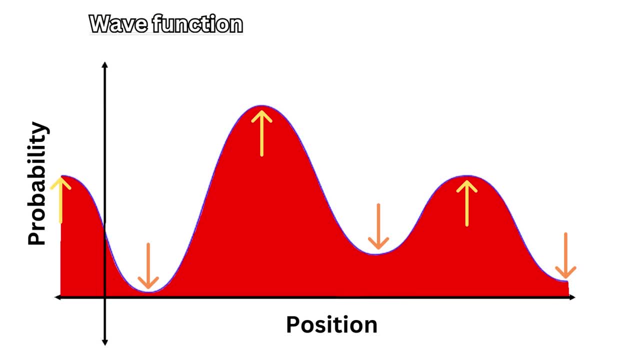 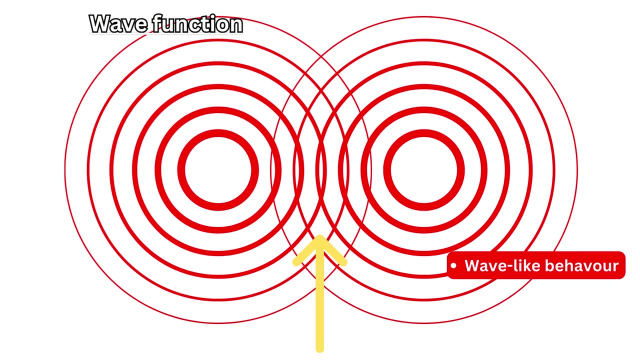 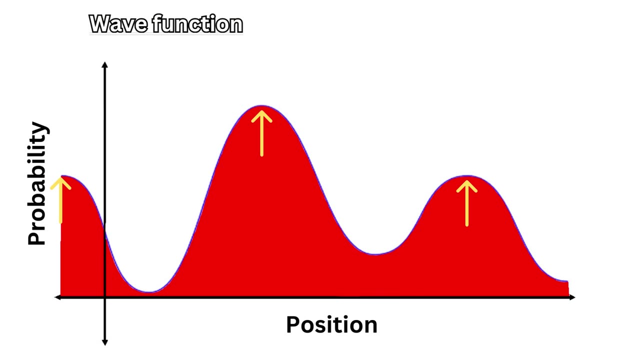 of higher or lower probabilities of locating the particle at various locations when they overlap. this is referred to as wave-like behavior or quantum interference. it implies that the overlapping waves of possibility might either increase or cancel out the likelihood of detecting a particle at specific locations. as a result, patterns are developed showing 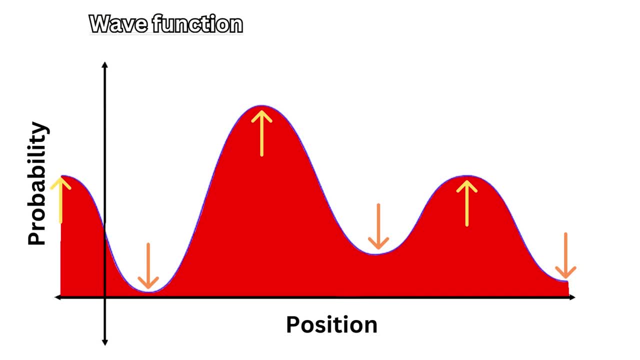 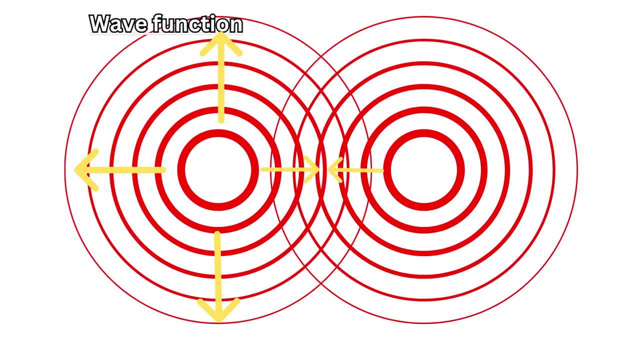 where the particle is more and less likely to be detected. this means that the wave function itself behaves like a wave, propagating and interacting with other waves of possibility. one of the explanations for why the quantum world operates differently from the familiar world of ordinary objects is this peculiar and perplexing aspect of quantum mechanics. 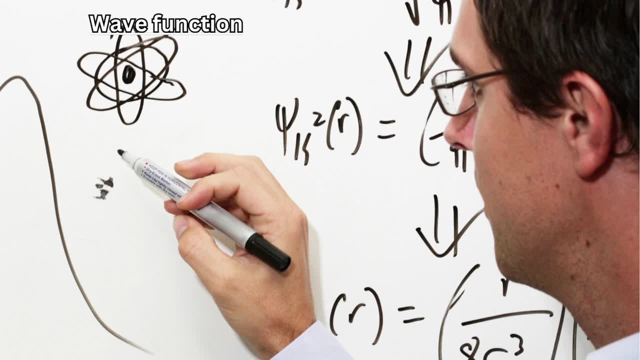 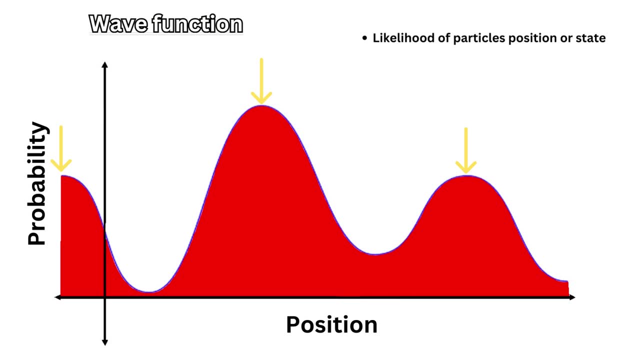 however, we must keep in mind that the wave function is a mathematical equation that calculates the likelihood that a particle would be found in various positions or states. it is a method for predicting and comprehending how sub-atomic particles like electrons or photons behave in the quantum environment. you could compare wave function to stating something like: 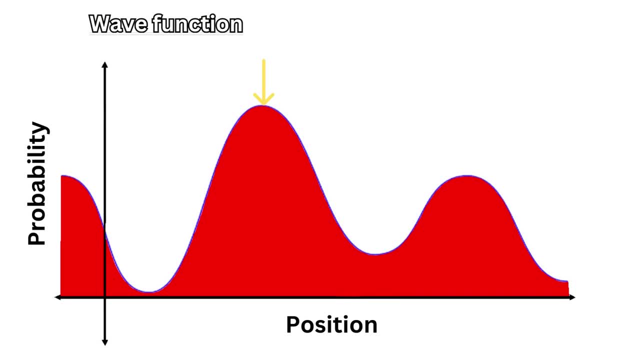 this, there's a higher chance of finding the particle here and the lower chance of finding it over there. before being measured, a particle's behavior is characterized by its wave function, which is a superposition state. so what superposition basically means is that it appears as though the particles are simultaneously existing in a number of possible states.